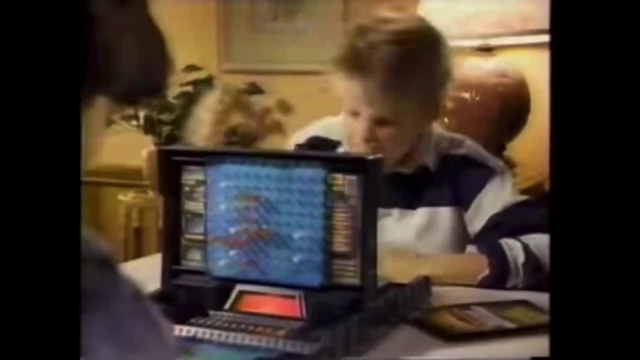 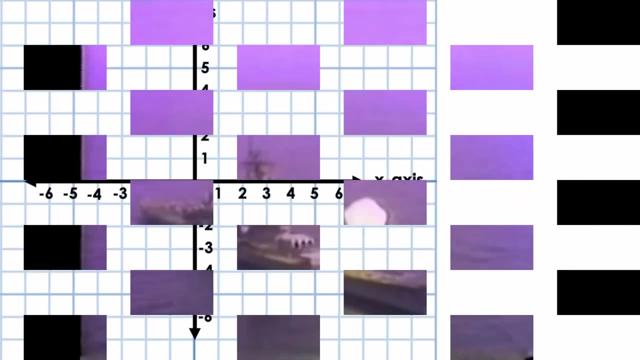 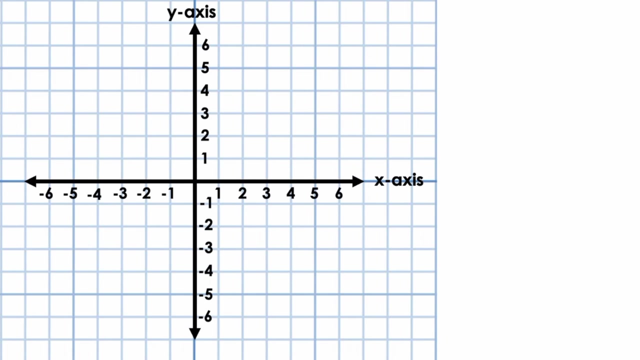 on the coordinate plane. The location or coordinates of any point plane can be identified using a pair of numbers. The first number in the pair identifies the point's location along the x-axis. The second number in the pair identifies the point's location along the y-axis. There is a special format for writing the coordinates Each number. 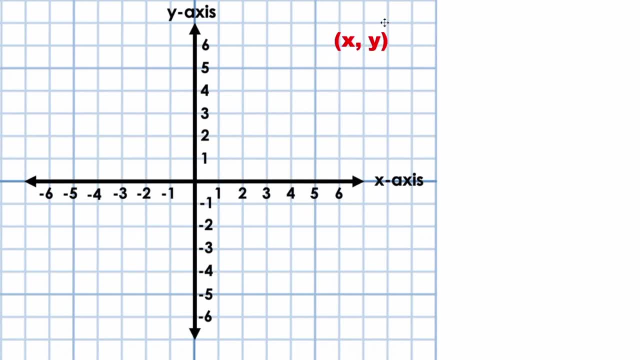 is written in side parentheses, separated by a comma. The first number listed is always the x-coordinate. Remember, this number refers to the point's location along the x-axis. Pretty cool, eh. The x-coordinate is along the x-axis. The second number listed is always: 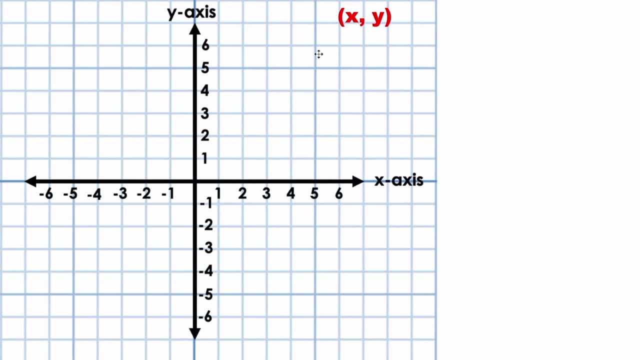 the y-coordinate, Remember. this number refers to the point's location along the y-axis. The y-coordinate is along the y-axis. You may also hear the coordinates referred to as an ordered pair. This is because the coordinates are a pair of numbers that are always listed. 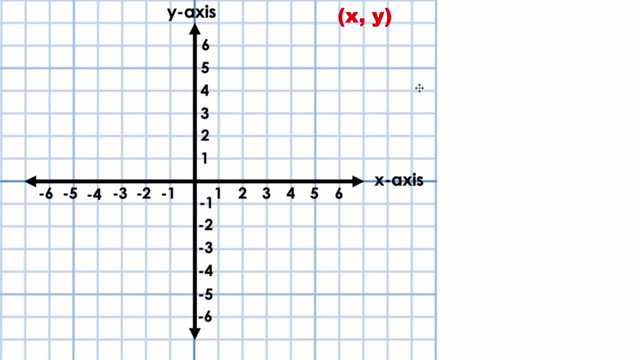 in the same coordinate, In the same order: x and y. If we know the x and y coordinates for any point, we can locate that point on the coordinate plane. There are four steps that you can take to plot any point on the coordinate plane. To show this, let's plot the point with the. 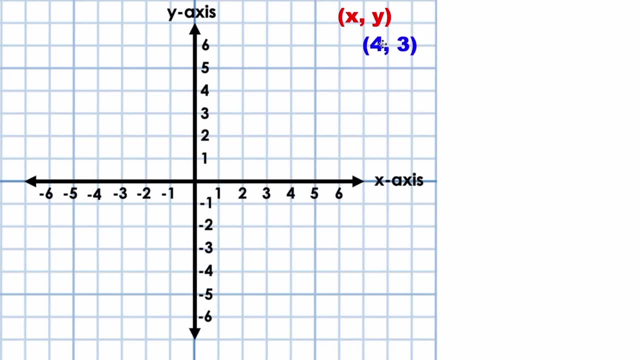 coordinates 4 on the x-axis and 3 on the y-axis, On the right side of your screen. I'm going to list four steps for success. First, start at the origin. Remember the origin is the point where the x and y axes intersect. 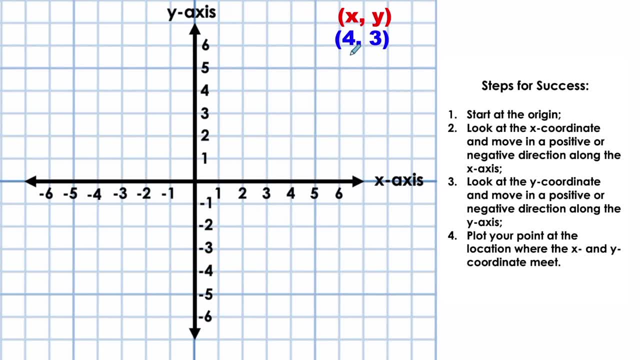 Second, look at the x-coordinate. It's the first coordinate in the ordered pair and move in either a positive or negative direction along the x-axis. In this case we have positive 4.. So we're going to move positive 4 on the x-axis. 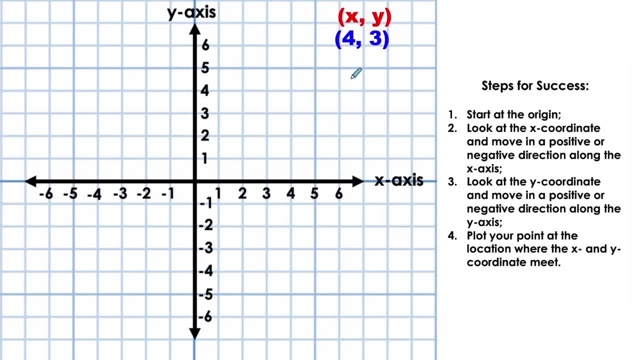 The third step is to look at the y-coordinate. Remember, it's the second coordinate in the ordered pair And you're going to move in a positive or negative direction along the Y-axis axis, In this case, we have positive 3, so we're going to move up positive 3 spaces. 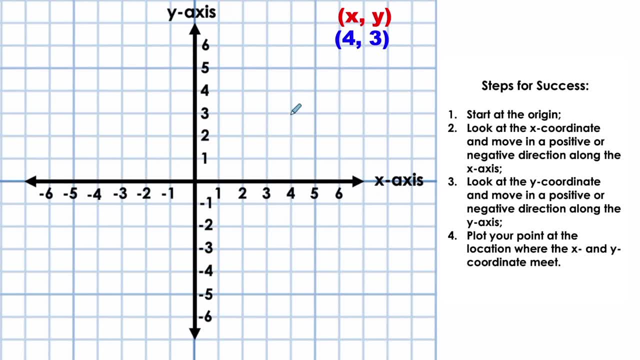 Your fourth and final step is to plot your point at the location where the x and y coordinates meet. Right here is our point 4 on the x and 3 on the y axes. You might have already noticed that the coordinate plane is divided into four. 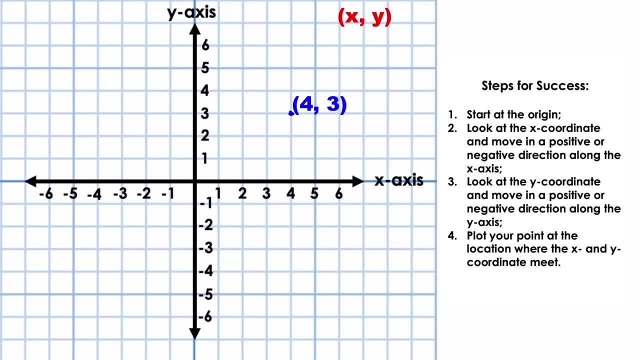 sections. Each of these sections is called a quadrant. The first quadrant is identified using the Roman numeral 1.. Every point located in the first quadrant has a positive x-coordinate and a positive y-coordinate, just as we saw with our example. The remaining quadrants are numbered moving in a counter. 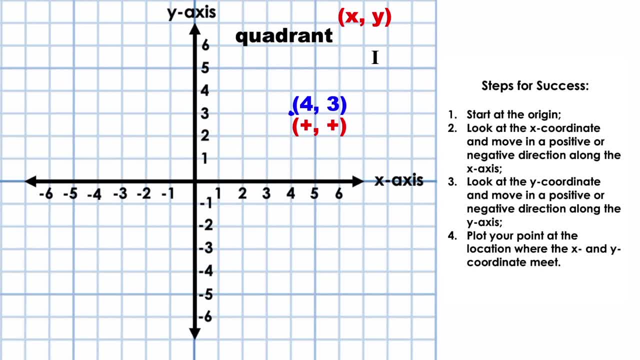 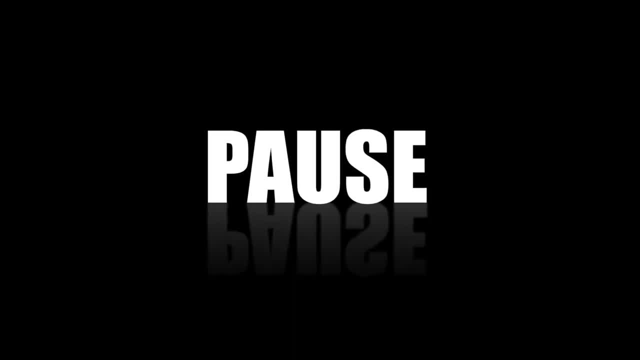 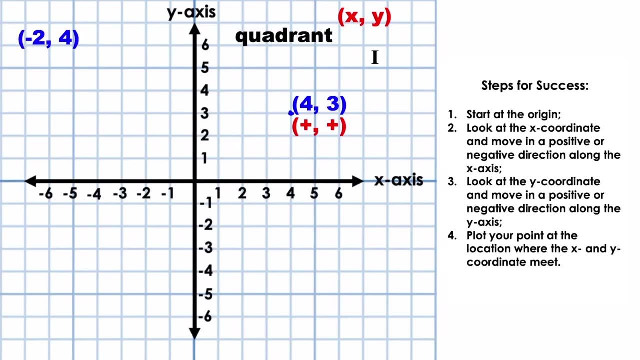 clockwise direction about the origin. Pause the video and take a moment to plot the point located at coordinates. How did you do? Let's take a look To plot the points. we start at the origin and we look at our x-coordinate. so we're going to move. 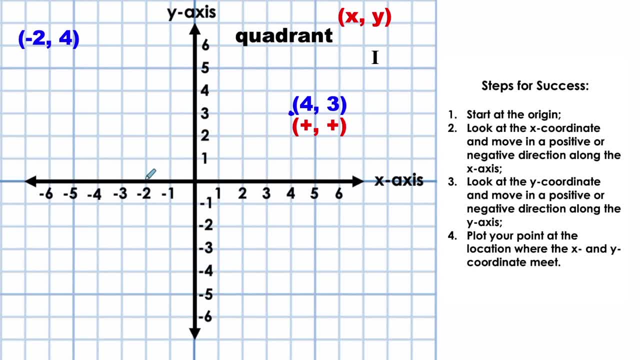 negative: two places along the x-axis. We then look at the y-coordinate, which is positive, 4, so we're going to move four places in a positive direction on the y-axis And our point is going to be right here. So this point is negative: 2, 4.. These 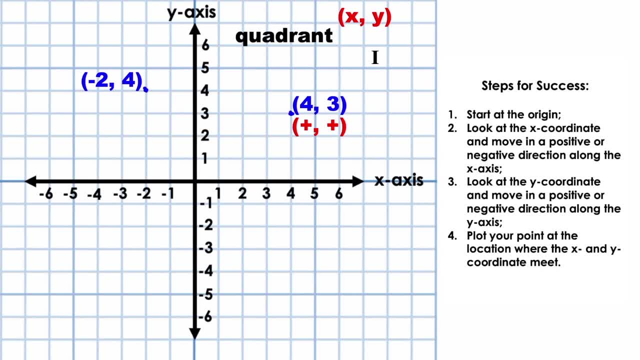 points is located in the second quadrant, again identified using Roman numerals. Every point located in quadrant 2, will have a negative x-coordinate and a positive y-coordinate. Take another moment to plot the point with coordinates will be located in the third quadrant To plot the points at coordinates. 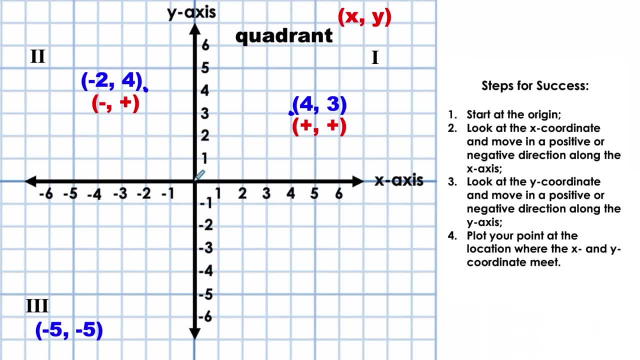 we start at the origin and we move negative 5 places along the x-axis and then negative 5 along the y-axis. So our point is right here and this point is: As you can see, every point in the third quadrant is going to have a both negative x and y coordinate. Let's take a 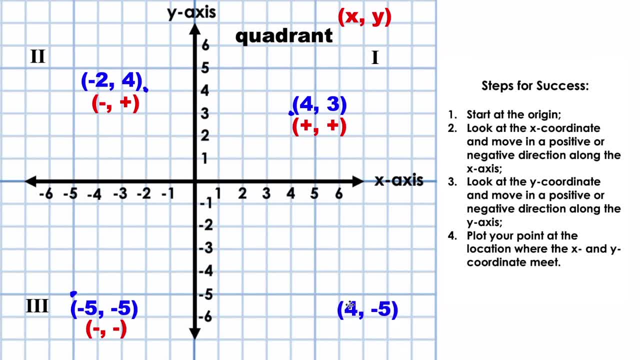 final moment to plot the point with coordinates. Once again we start at the origin and we look at our x-coordinate. The x-coordinate is positive 4, so we move positive 4 on the x-axis and then we look at the y-. 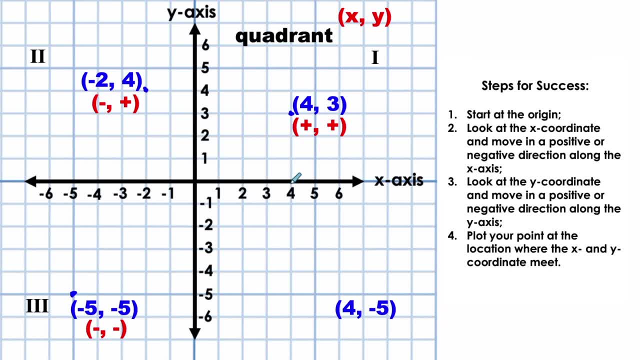 coordinate, which is negative 5, so we're going to move negative 5 on the y-axis and our the location of our point for negative 5 is right here, So we'll label this and finally, as you can see, any point located in quadrant 4 is going to have a. 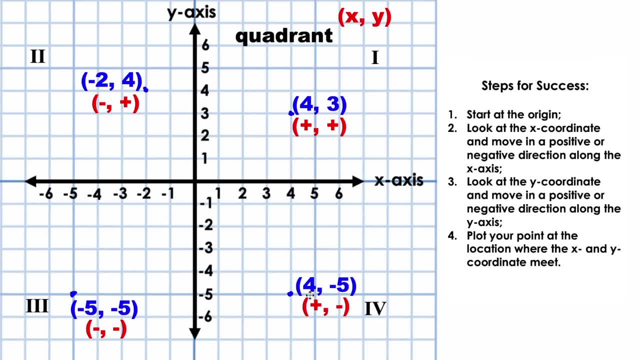 positive x-coordinate and negative y-coordinate. Sometimes you will locate points that are not in any one quadrant. This is because the point is located on either the x-axis or the y-axis. For example, the point is not in quadrant 1 or in quadrant 2.. 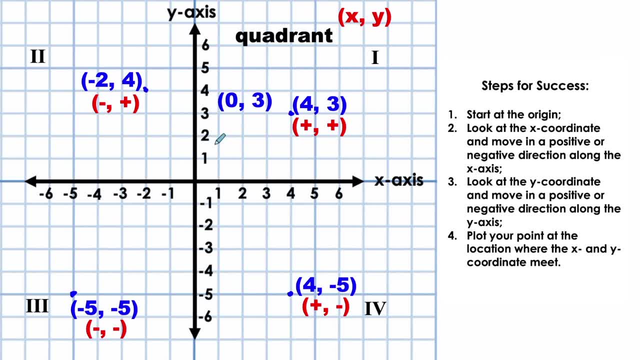 It is located on the y-axis. We don't move either in the positive or negative direction on the x-axis because our first coordinate is 0, but we do move up positive 3 on the y-axis. so the point is right here, The point located. 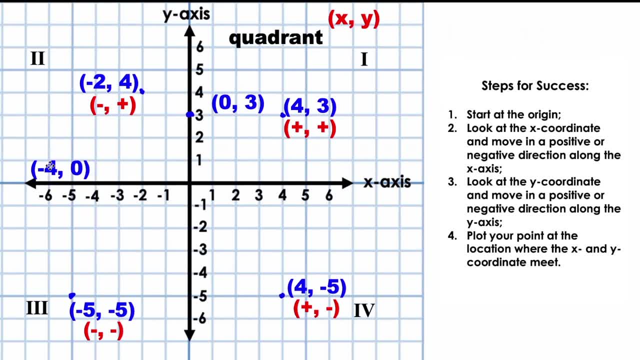 at coordinates negative 4, 0 is not in quadrant 2 or in quadrant 3.. It's located on the x-axis, Starting at the origin. we're going to move negative 4 along the x-axis, but our y-coordinate is 0, so we're not going to move up or down on the. 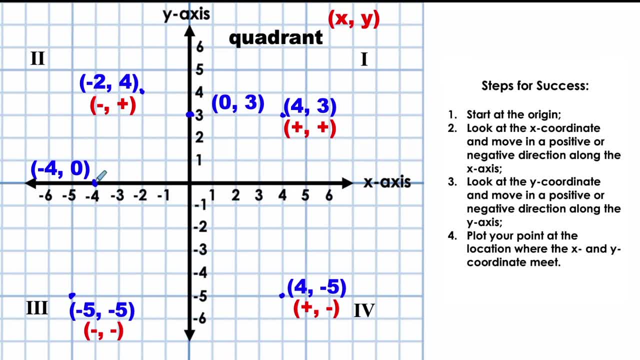 y-axis. So our point lies right here, at negative 4 on the x-axis. As we can see, any point on the coordinate plane will lie in one of the four quadrants on the x-axis, on the y-axis or right at. 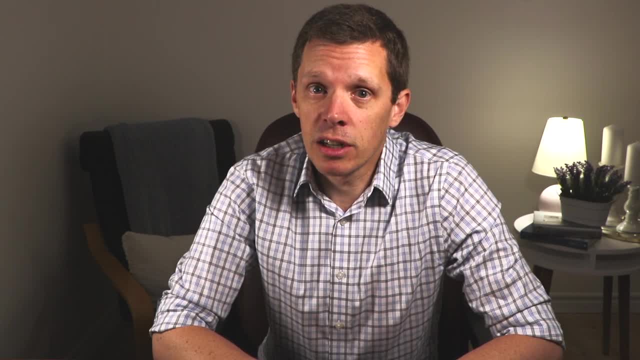 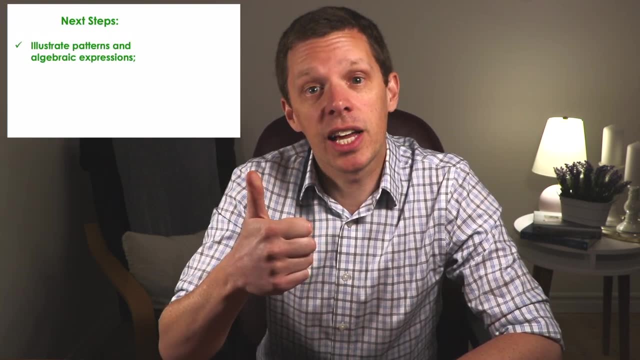 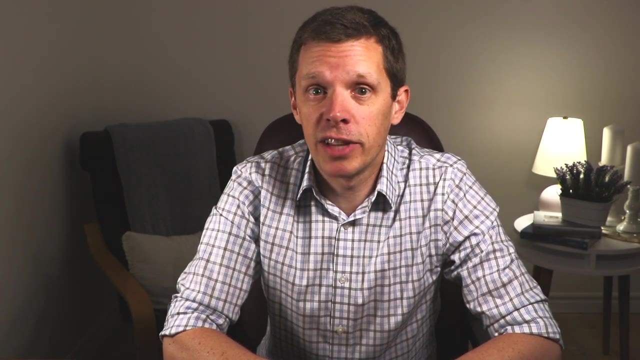 the origin. So where do we go from here? Well, a thorough understanding of the coordinate, or Cartesian plane will help you illustrate patterns and algebraic expressions, draw polygons and transform polygons using dilations, translations, reflections and rotations. All that is.